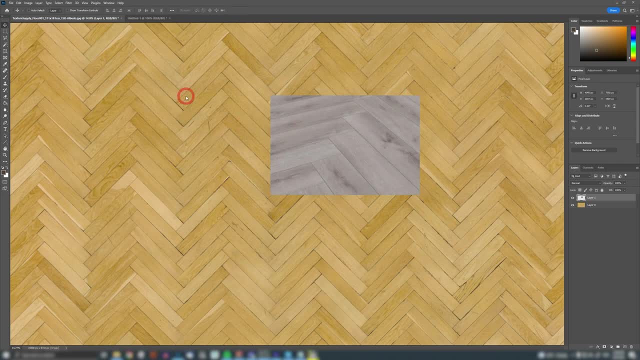 And now you can clearly see the color differences. So, before we proceed, always make sure that your image is in 16-bit. As you can see, this image is in 8-bit. It says here: RGB 8.. So go to image mode and just switch it to 16-bit. Now, why is this important When you switch it to 16-bit? 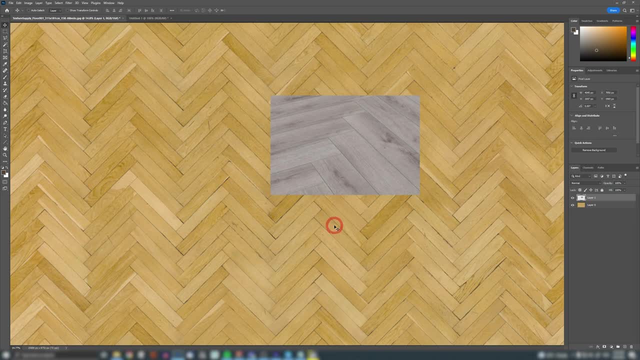 your texture will not become a 16-bit image. It will still be 8-bit, But we're going to be adding a lot of color correction, like hue, saturations levels etc. But all of these color effects will be processed through that 16-bit. And that is super important because if 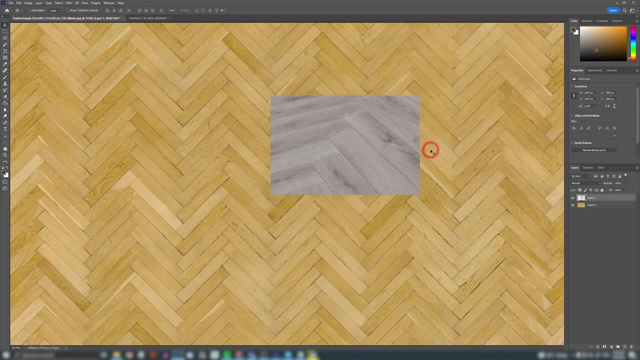 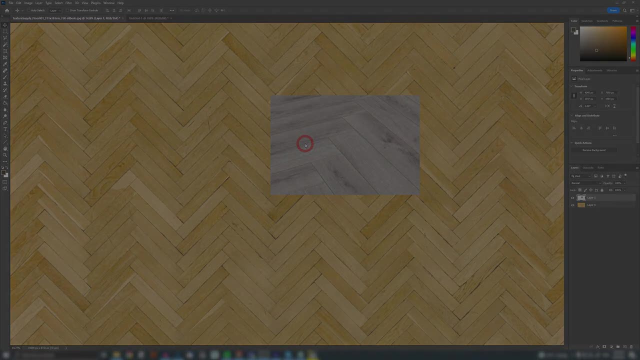 you're going to be doing heavy color corrections, you will avoid a lot of bending effects and all the negative errors which can destroy your image. Now I like to separate my color corrections into three segments: Light intensity, saturation intensity and color tone. Let's start with light intensity. 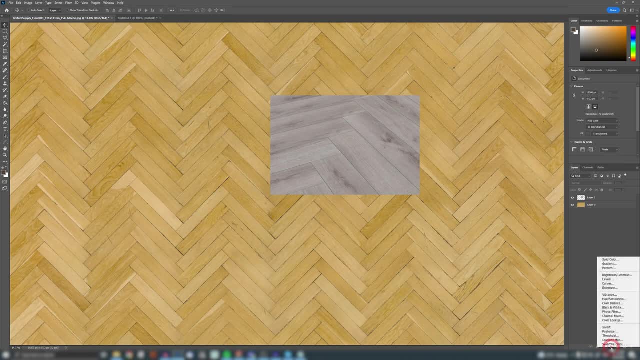 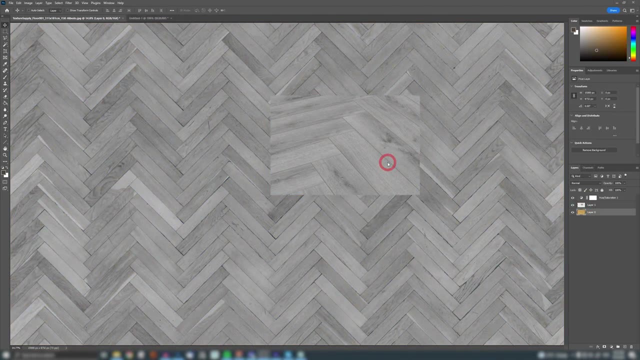 So to determine the light intensity in your texture, you want to add adjustment layer hue saturation, on top of these both layers and just drop the saturation to zero. Now, at this point you can see if your background image is lighter or darker than your reference image. that's the 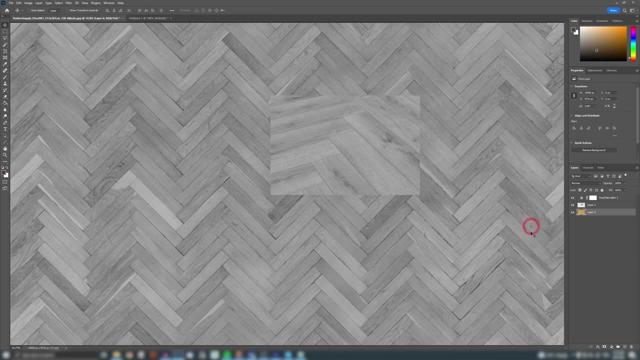 light that you need to correct, And I correct that light with levels. So let's add levels to the whole story. Now, the levels must be in between these two, because you don't want to affect this image, because you don't want to affect the overall image. Now, if you move the middle slider here, Now, this is the 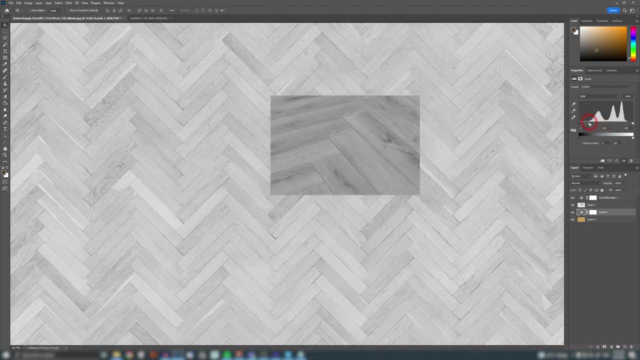 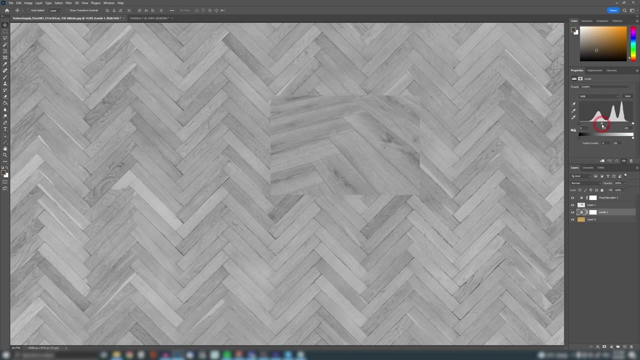 gamma. If you move that gamma up and down you will see how our reference image is sticking out more and more. Let's just try to move gamma a little bit up to kind of try and match overall tone of the image. Now I'm kind of satisfied with this. Let's just drop the dark parts a little bit just. 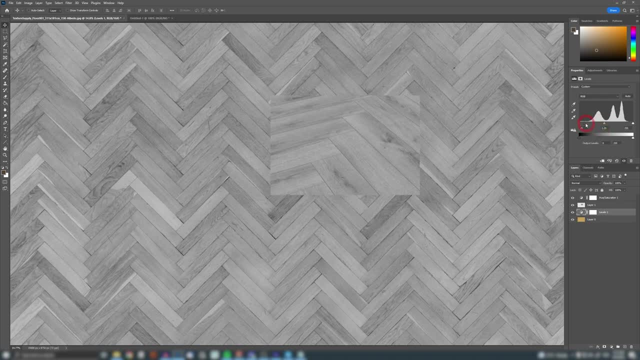 a touch And we can maybe bring up the lightness here a little bit. Maybe this, something like this: I'm satisfied. Now from this point you need to check if your lightest parts and your darkest parts kind of match, So you see the lightest parts here, darkest parts here. So you want to kind of get an 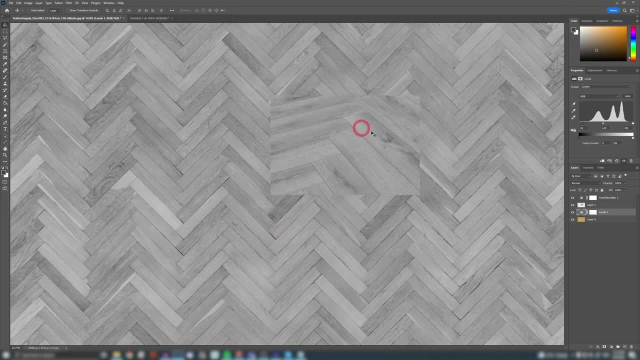 overall feeling if you see those elements matching this reference image. If they do, your lightness part is done. Now let's switch to saturation intensity. From this point, we can safely turn off hue and saturation here, and we're gonna introduce a new adjustment layer and that's gonna be hue. 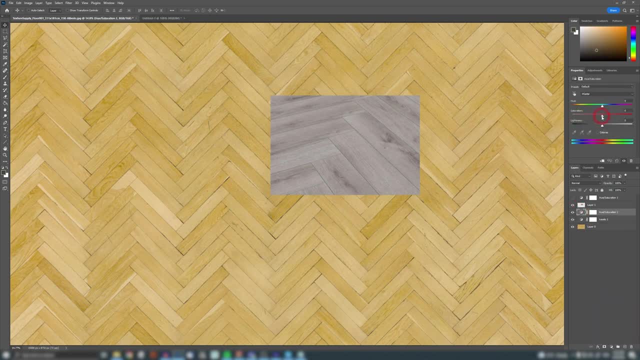 saturation. So let's go ahead and add a new adjustment layer and that's gonna be hue saturation. So if I click here and go to my saturation levels Now, we need to reduce the saturation so that the saturation matches our reference image. As you can see, our main texture is highly saturated. 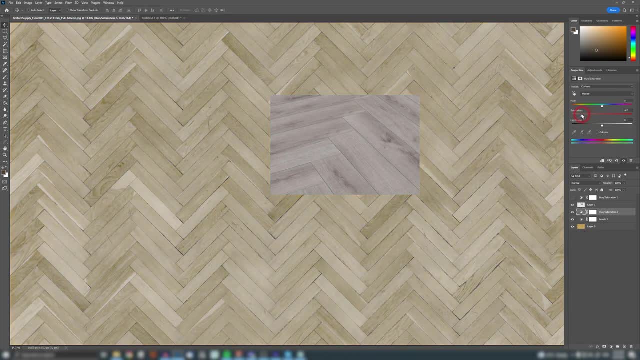 comparing to the image that we have here. So let's drop this down to something like: maybe that's too much. Let's say something like this: I think the levels of saturation here kind of match and we are roughly done with our saturation intensity. Now let's move to the color tone. So for color tone. 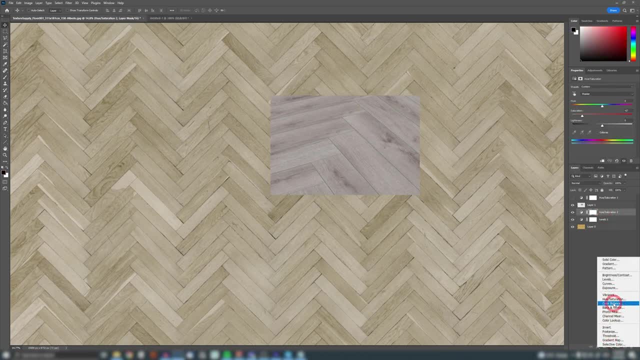 we're going to add an additional adjustment layer and that's going to be color balance. So with the color balance you freely want to experiment with these three sliders. You can even go a little bit in depth and try to match the shadowy parts, the highlight parts. But for 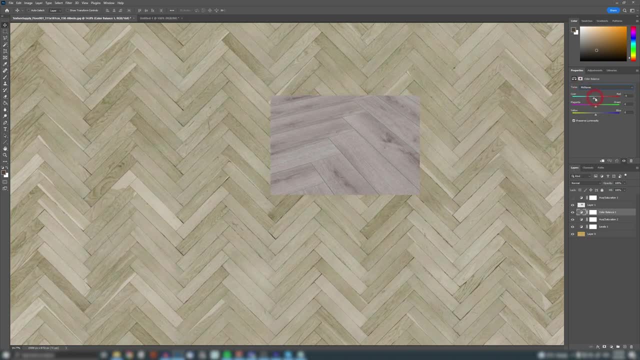 this example, we're going to stick to mid-tones. So if you just move it left and right, you will see when it kind of starts to match closely to this image. So what I? since I moved it to the right I kind of noticed: yeah, this image has a bunch of reds in it, So maybe this is a good. 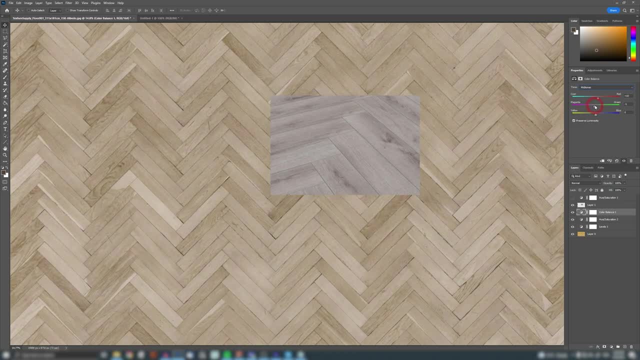 way to go. So let's go with the second. So the second kind of doesn't sit anywhere. So I'm gonna keep it close to zero and let's move this slider. Okay, so I see, if I go to the blue side, that we are. 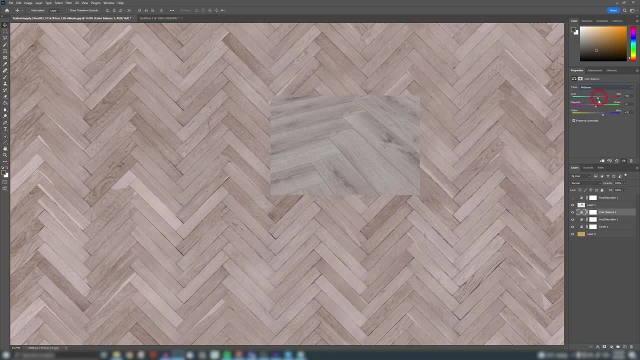 getting closer. So let's kind of crank that blue up and try to tweak these two. Let's move this back, since I have too much red now. Move this a little bit to the greener side, Maybe something like this, and add a little bit more blue here, for example, And now you can see that we are. 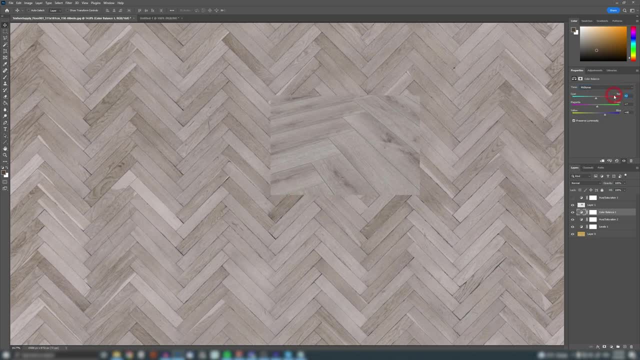 very, very close to the color. So let's just do a few final tweaks. I think there's maybe a little bit too much red going on, So let's keep this to zero and this is okay. And I in general, I think this is pretty much done. And let's view our texture from the close-up, So if we zoom in, Okay.